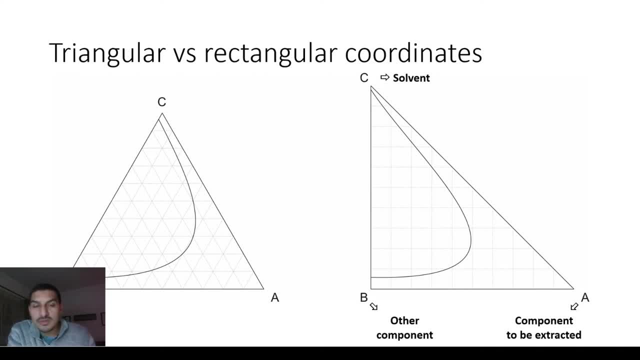 hello everybody. we're still talking about the liquid-liquid extraction and last time we talked about the phase diagrams and the coordinate system that we are using and we said that we are going to use the rectangular coordinates because it makes it easy for us to extract and put data on the diagram and 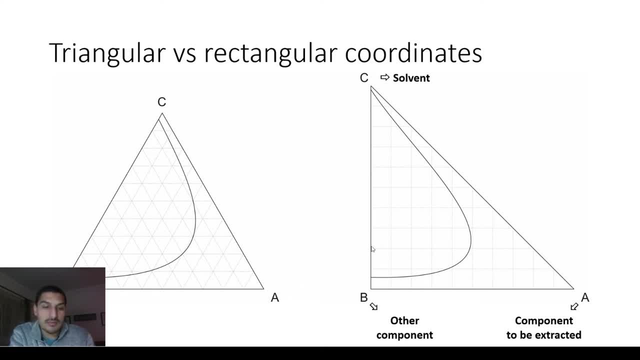 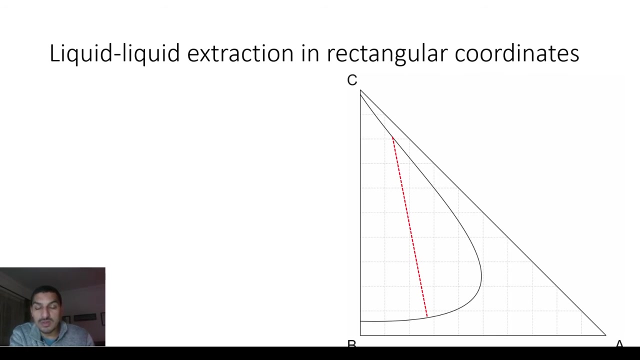 then it is for the triangular coordinates and this is what we ended up saying: that this corner C represents the solvent, B represents the component that I am interested in getting in pure form and A is the impurity that I want to extract. and before we start and do the calculations and see what we are gonna, 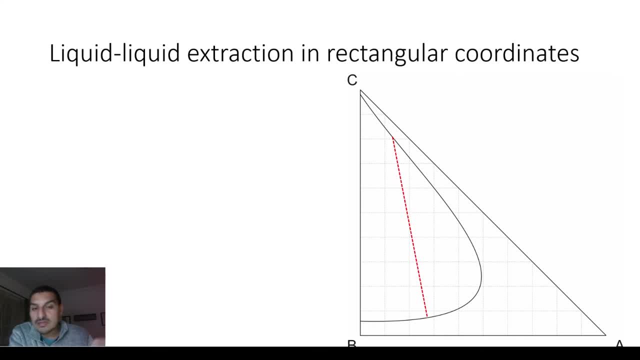 do with the phase diagram. let's let's get to know its components more so. the phase diagram simply contains this line, which is the equilibrium curve. the equilibrium curve splits the region, or the the area, into two regions: the two-phase region, which is the region that splits into two phases. 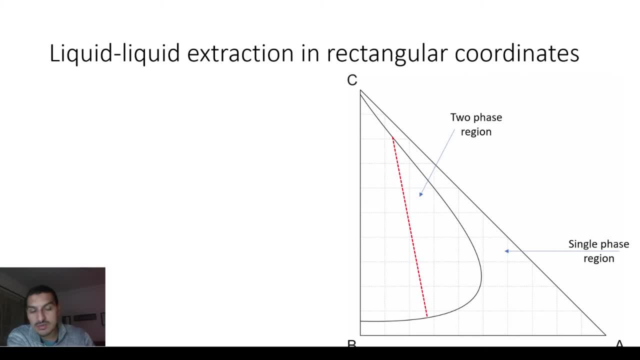 spontaneously, and the single phase region, which is the homogeneous phase, and for the, the two-phase region, it contains what we call the tie lines. that tells us what is the equilibrium relation. so this tie line cuts, or it intersects here in a point and here in a point, and these two points are: 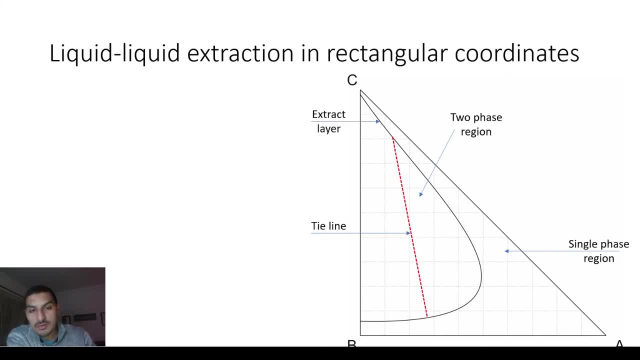 in equilibrium, the top part of the equilibrium curve we call it the extract layer and the bottom part is the raffinate layer. then when we do extraction for, let's say, single stage, we have the mixture that I want to purify. I will. I have the solvent V2 that I know that I'm gonna use to do the separation. 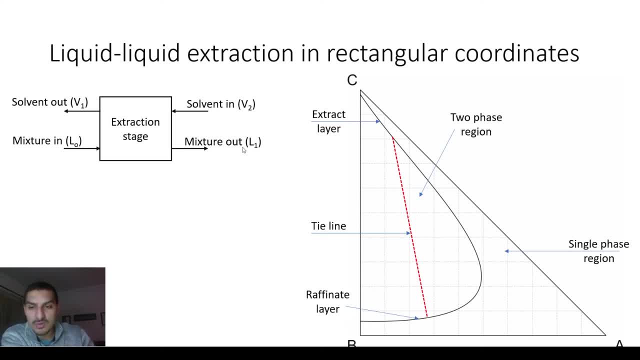 or the extraction. I know that the prod there were two, two. there will be two outputs: the solvent, after getting a out of B or subtracting it out of B, and the mixture that is gonna be having less amount of a or less percent in a, and this is what we want to do and the aim of the work that we're. 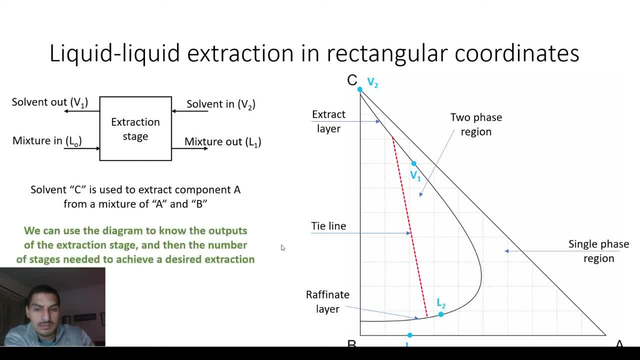 gonna do is to use the phase diagram to know LV1 and L2 as compositions and flow rates. I know that the V1 will lie on the extract layer and L2 will lie on the raffinate layer, but I don't know exactly where. so this is. 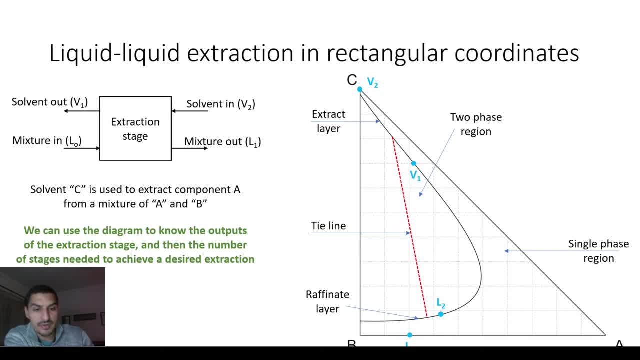 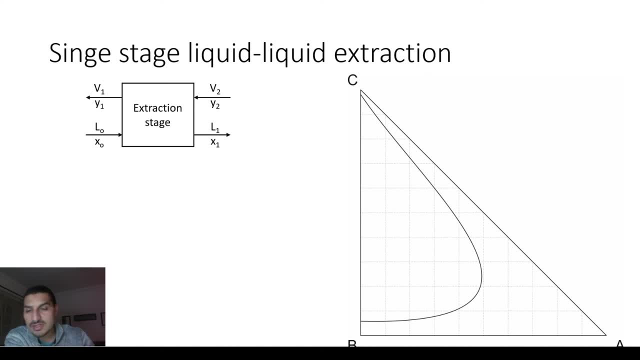 what we're gonna do in the this video today. so let's go ahead and start with the simple case, which is the single stage liquid liquid extraction. for the single stage, I know that L node and X node are contacted with VY or the or V2, and X node represents the composition of the L node or the liquid. 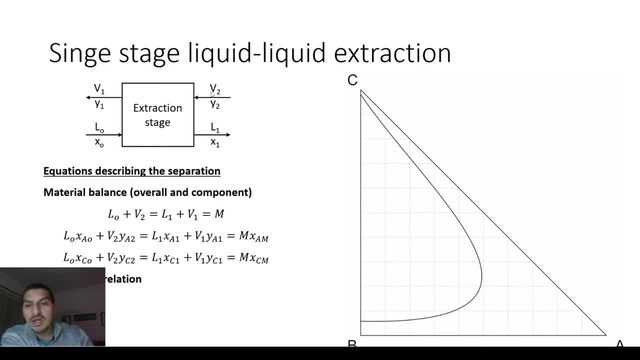 stream Y, node Y2 represents the composition of V2 and the same for Y1 and L1. so this system can be suppressed by the material balance, which is the overall material balance. L node plus V2, which, is very simple, equals V1 plus L1. 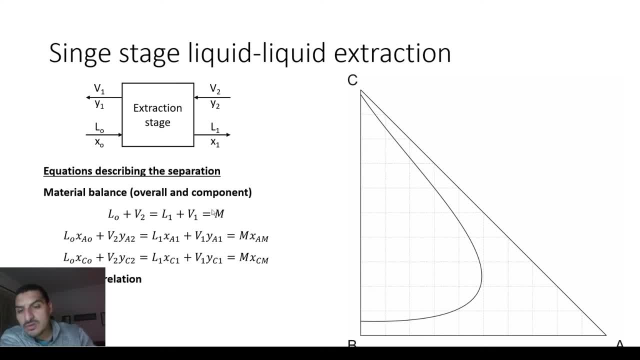 pretty straightforward and I call: the sum of these two is M. I can apply this on a component A and C and we usually do the component material balance on A and C because they are easy to put on the phase diagram. B is kind of difficult because it is. 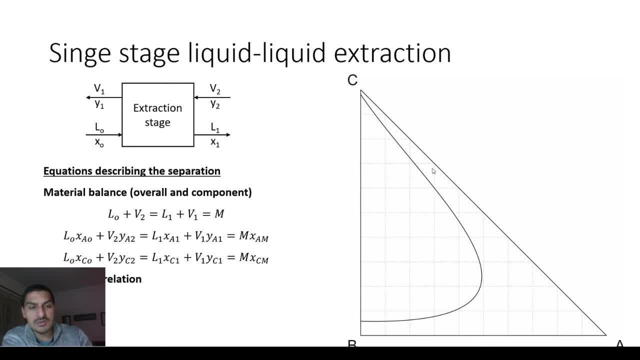 parallel. the percent B or the constant percent B is parallel to the hypotenuse, which is is not as easy, and that's why we use A and C, and actually we only get three equations because we have three components. so this overall, with the two component material balance equations, will be more than enough. so now let's. 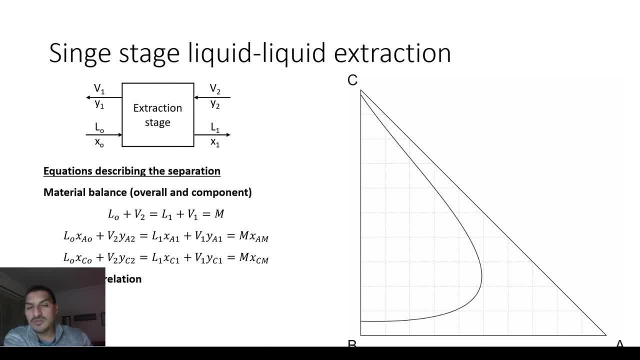 see what are the information that we need to know, to know what the G Vegeta Dong, which is the common Co2 sources that we know, and how we can use the thing that can to do this calculation. so my goal now is to know what will be the output, the amount and 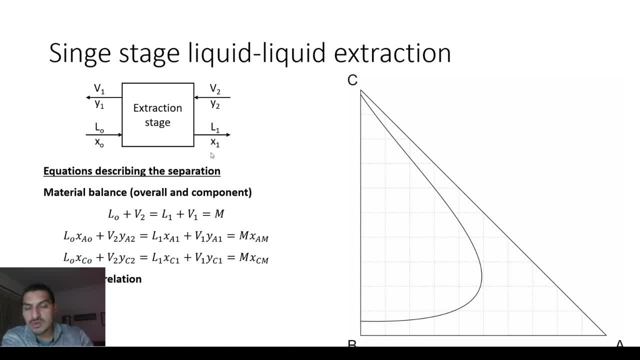 the concentrations of y1 and of every one and L1 and the composition to it, which is y1 and X1. this is my goal now. so first we we need to know what the information or without information that we know. so you know, D amount of the. 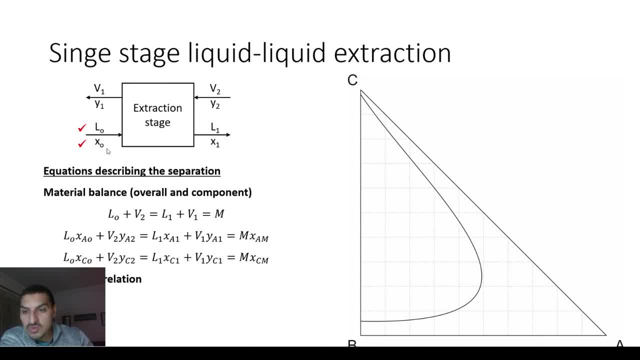 liquid feed and the composition. so after taking this, this will enable me to know where exactly i'm gonna put it on the diagram and this will help me do the lever arm principle calculations. the same here for v2 and y2, so i know the feed that. 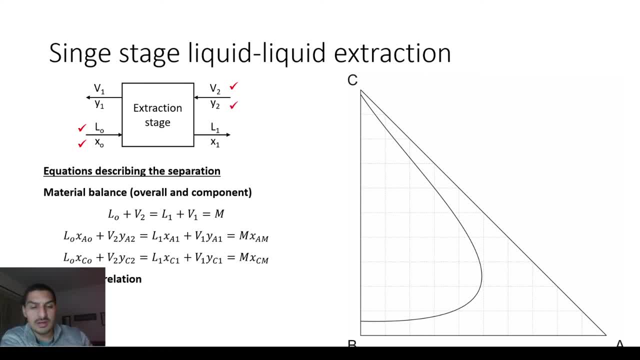 i'm putting for the solvent and for the fresh feed, and to put this on the diagram, usually the feed is a mixture of a and b. it doesn't contain any amount of solvent, so it's going to be somewhere here. and for the solvent, it's going to be here as a pure solvent. and now let's, let's see. 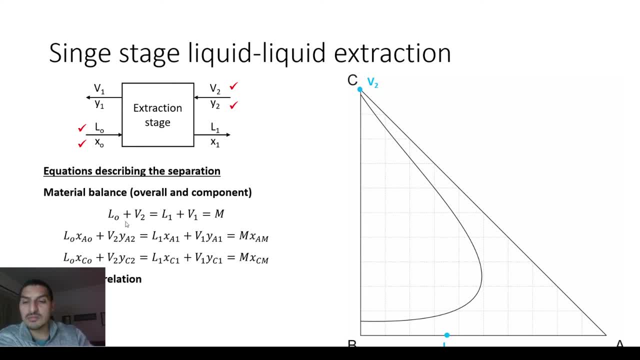 this equation is a mixing of two streams, which is kind of like this. so it's it in principle. i know from the physics of the process that l1 and v1 are going to be separated from each other, but the equation as an equation or a straight line that we are. 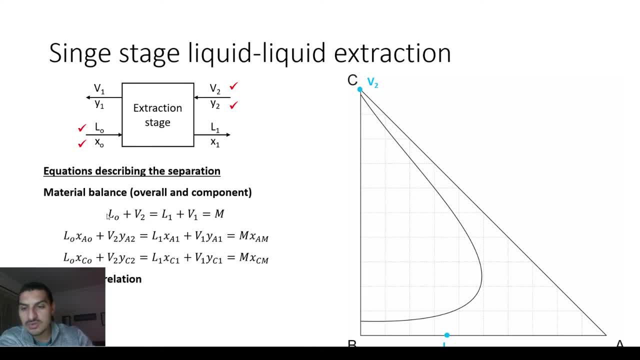 going to be separating from each other, is going to be separated from each other, and so i'm going to draw on the diagram. is is exactly like this. so so these two tell me that these two lines- line connecting l node and v2 and line connecting l1 and v1, and these two lines will intersect at point. 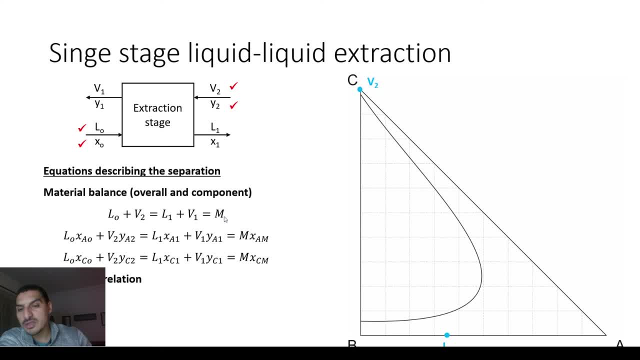 m and from the lever arm principle i can get all the information that i want to know. so i have v2 and l1. i connect them. it gives me the operating line. i can locate the point m from the lever arm principle. i know l node as an amount and v2 as an amount from the amount. 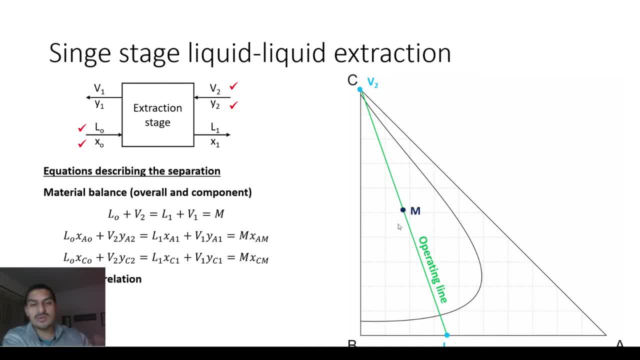 i can tell exactly where point m is, which is going to be somewhere here, depending on the amounts of both, and then i check where is the tie line that passes by point m. i use the tie line and intersect the raffinate layer and extract layer to get v1 and l1. so it's pretty simple and straightforward. 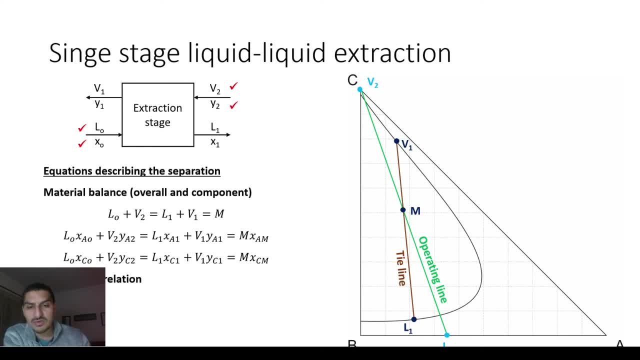 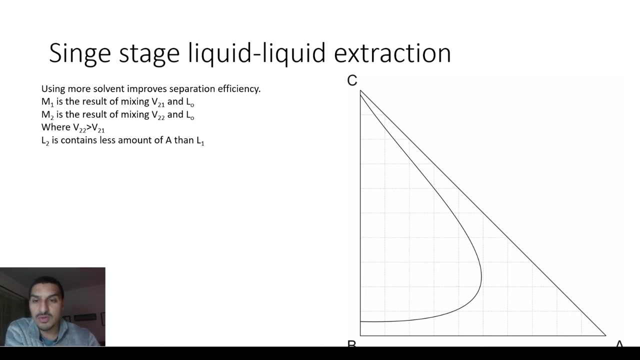 actually to do these calculations or the the graphical solution for a single stage, but there are a couple of points that i want to highlight just to to make this more useful and get the most information out of this. so, let's say, i have the same, the same mixture that i want to purify. 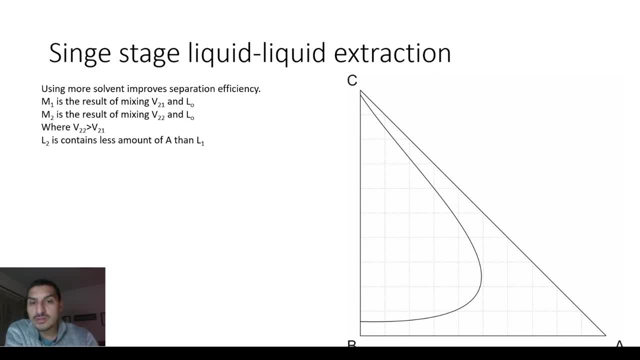 and i use two amounts of solvents: one. one time i'm using a small amount of solvent and the other time i'm using a large amount of solvent. so the, the simple logic, without even looking at the equations or looking at the, the diagram, the simple logic tells me that i use more solvent, then i get more extraction. so i'm 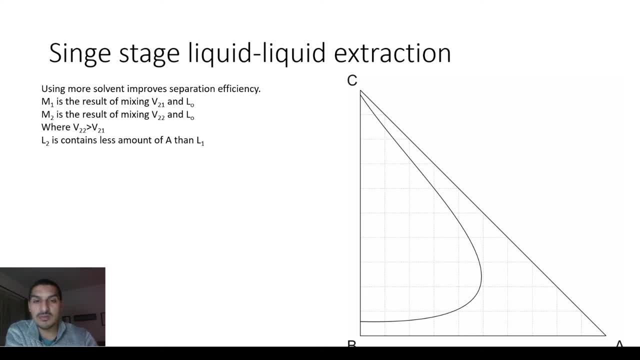 expecting that the, the mixture that i'm feeding to the extraction process, will exit with a smaller amount of a. then it will do with a small amount of solvent. so this is the simple logic and this is what we're gonna check now. so i i'm i'm putting the same feed, l node and v21 is the amount of. 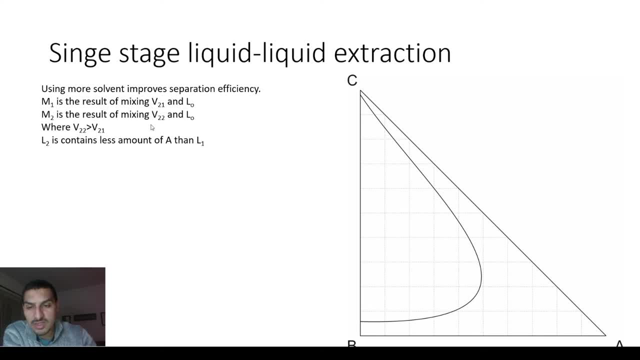 solvent that i'm using, which is the small amount, and v22 is the amount of solvent that i'm using, which is the great amount. and i tell you that v22 equals or is bigger than v21, and i'm expecting l2, which is the output of mixing the feed with the v22, to have less amount of a than l1, and this is 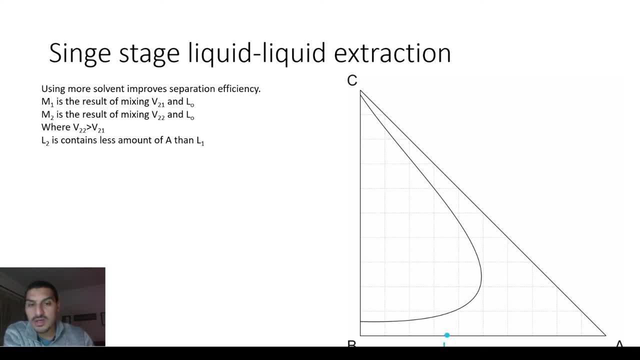 what we're gonna see from from the graphical solution now. so i'm locating l node, i'm locating from the line i can, and from the amounts of v2 and or v21 and l node i can get m1, and from the tie line i can get l1 and v1. the same thing would would be for m2, but for for m. for the second case, 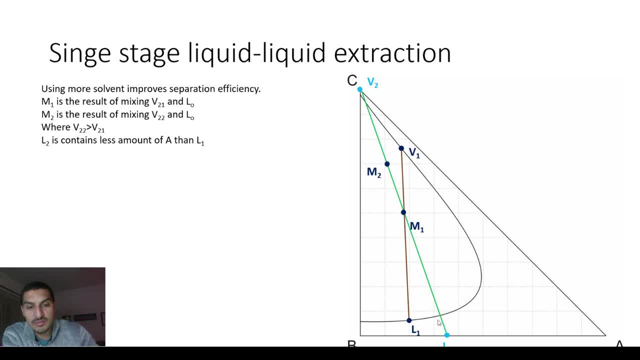 i have a larger amount of v2. that's why, from the lever arm principle, this distance would be larger. it's this. this will move upward a little bit, depending on the, the amount of v2, of course. that's why m2 is is here and then by connecting it with the 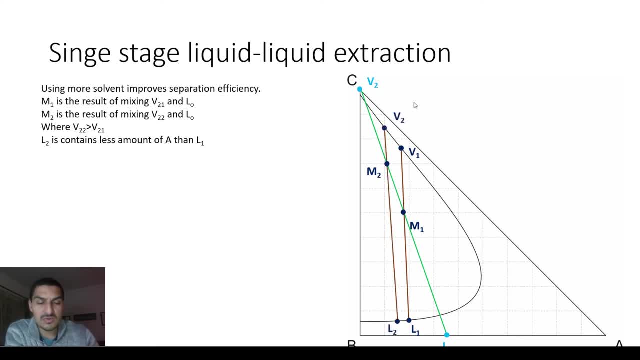 line and i'm going to get l2 and v2 as it is here, um on the diagram, um, and when you look now to compare l1 and l2- this is the point that we were looking at now- l2 contains less solvent, or less less a, i'm sorry, let's say, than l1, which is, yeah, this. this contains almost 15. this contains around 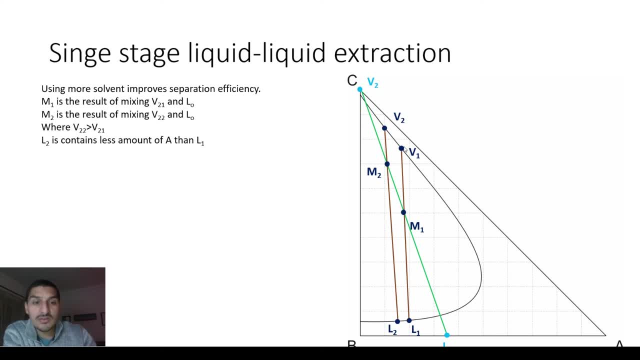 20 percent of a, which is great. however, if you check here, you will find that v1 contains more of a solvent than l1, which is great. however, if you check here, you will find that v1 contains more percent of solvent than v2. this is 10 percent, and this is around 17 or 18, which is not logical. 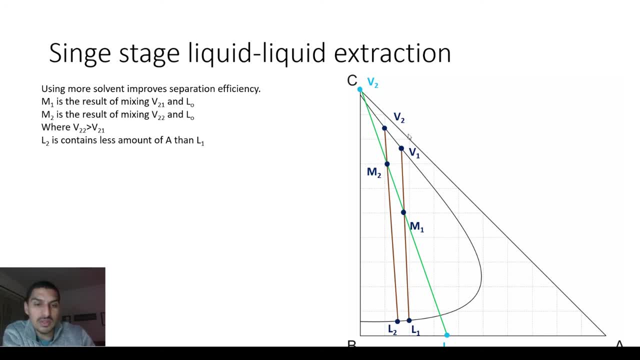 because i would expect that v1 would be um, not uh, or will contain more a than v2, right? i mean, v2 contains more a than v1 because it extracted more a than v1 did, and this is what i would expect, but this is not what the diagram tells me. um, and to understand this point, 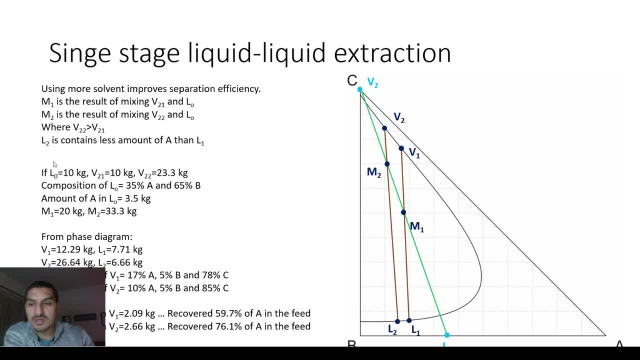 we need to put some numbers. so i'm i'm assuming that i'm using 10 kilograms of the fresh feed, um, and i'm using, in the first case, 10 kilograms of the solvent. in the second case i'm using 23.3 kilograms of solen, so it's it's around like 130 something percent. 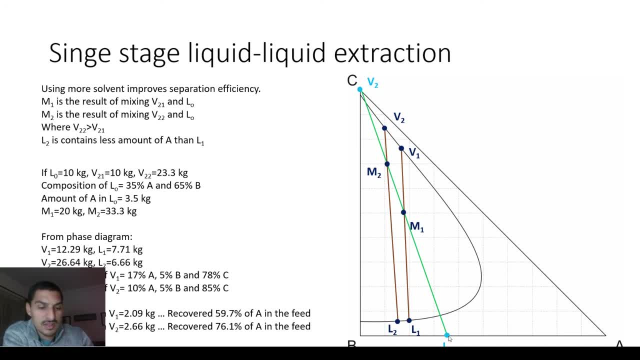 more solvent in the second case. i know from the phase diagram here that l node is around 35 percent a and this means that i'm using 33.5 kilograms of the a um. or there are 3.5 kilograms of a that i want to get rid of um and i can get m1 and m2 from. 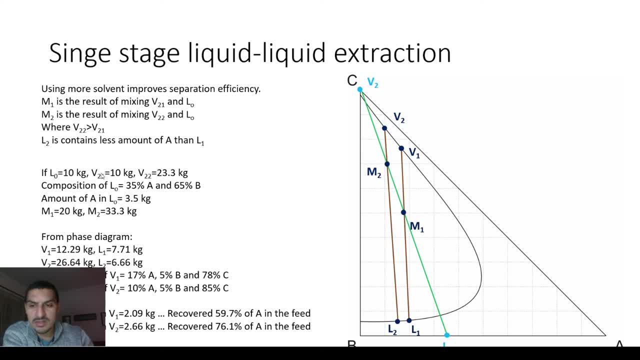 summation of these numbers, 10 plus 10 and 10 plus 23.3 um. and from the phase diagram now i can get some information. for instance, i can use this line, the first timeline, to get the amount of v1 and l1, as we mentioned before. i know the amount of m1 and i know this distance and this distance and 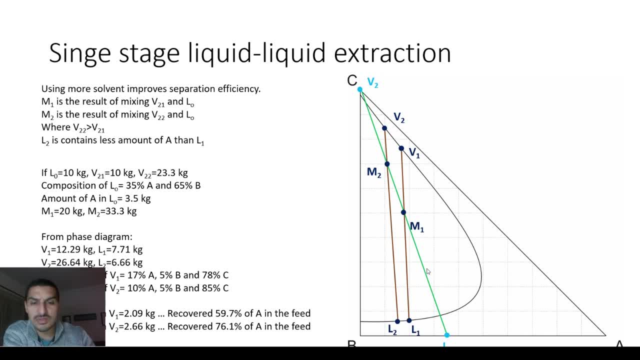 the total distance. so i can easily tell how much is l1 and how much is v1, and this is what i did here. the same thing i applied for the second timeline. i got v2 and l2 also. from the diagram i am able to get the composition of v1, the composition of v2, the composition of l2 and 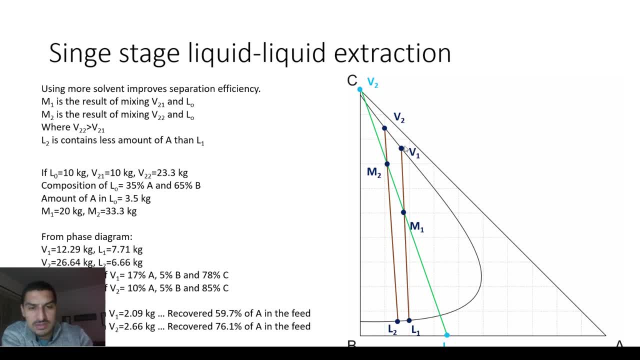 the composition of l1 and and usually, just to give you a hint, how to extract the, the data for, for instance, v, for v2, v1, i, uh. i usually get the two simple uh compositions that can be got simply from the diagram, which is a and c. so a is this is ten. 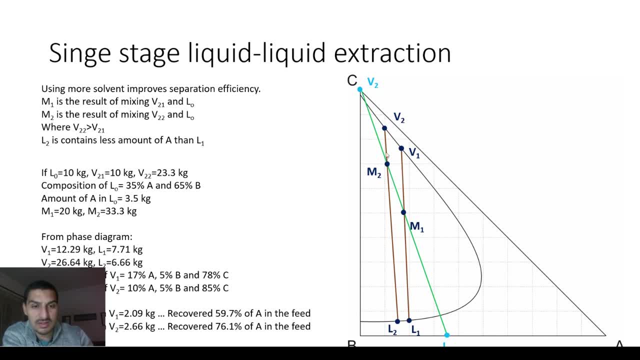 percent a. this is twenty percent a. this is the this dotted line and this dotted line. so this is going to be around 17 percent a, which is this, and for b, this is 80 percent, uh, 70 percent. this is 80 percent c, so this is going to be around 78 percent c, um, around something like that. so i know. 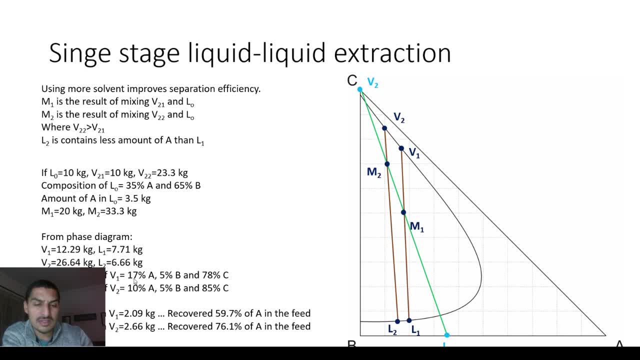 this is 78, this is 17, so the, the, the rest, uh, or the balance of the composition, would be the percent for b? um. and now let's see we have: v1 is 17 percent a and the amount of v1 is 20.29. 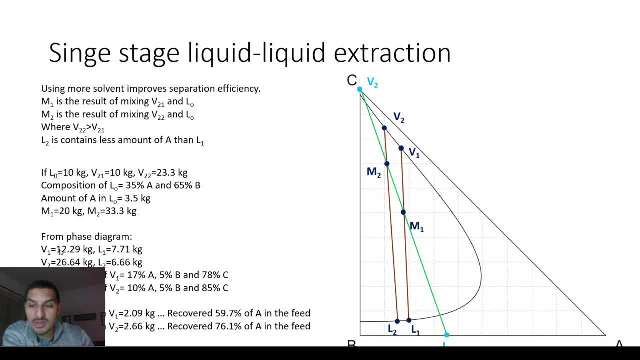 kilograms. so from these two, if you multiply 17 by 12.29, i'm gonna get 2.09 kilograms. so this recall or extracted around 60 percent of a from from that a entering with the feed. in the second case it has less amount of of a as percentage. it has 10 percent compared to 17 the first time. but 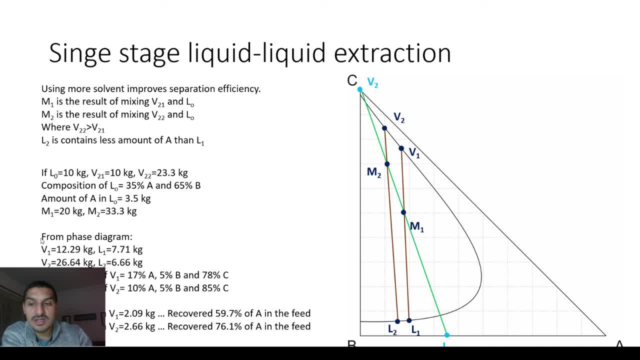 of the of the stream v2 is very large. it's- it's more than double the amount of v1, and this is because i'm using a lot of solvent in this second case. so when you multiply this 10 percent by the 26.464, you get 2.66 kilograms, which is extracting 76 percent of the a entering in the feed. so 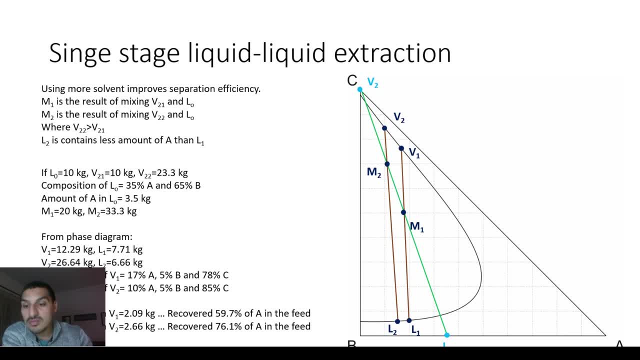 the. the percent a is lower because the stream is very, very large. so as a percent it's lower, but as an amount it's larger than than this case. so you would see that i i was able to increase the amount of a that i extracted by around 600 something, or it's like 570 grams. 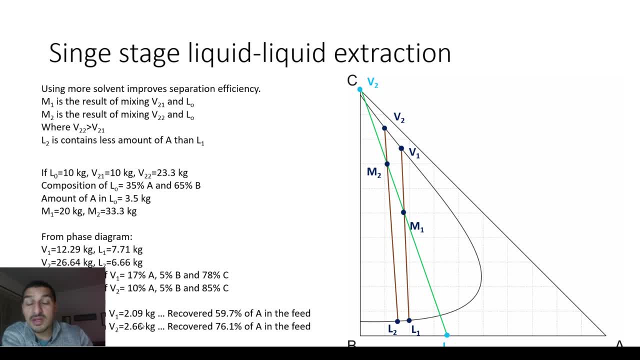 it's around half a kilogram, but by increasing the solvent. but i did this or achieved this by increasing the solvent by 130 percent, which is a great rate amount. this is not practical and it's not economical. the solvent costs money and it will cost you money for operating um the the unit by pumping, and then to do the separation to reuse it. 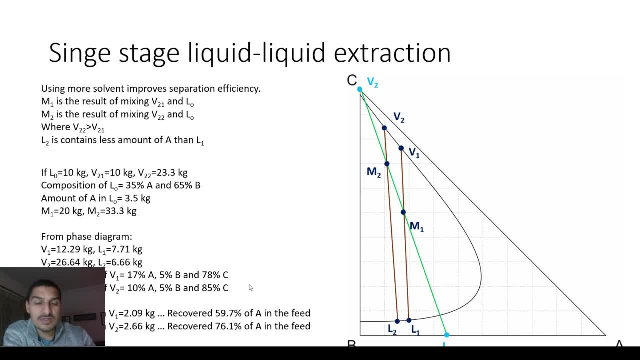 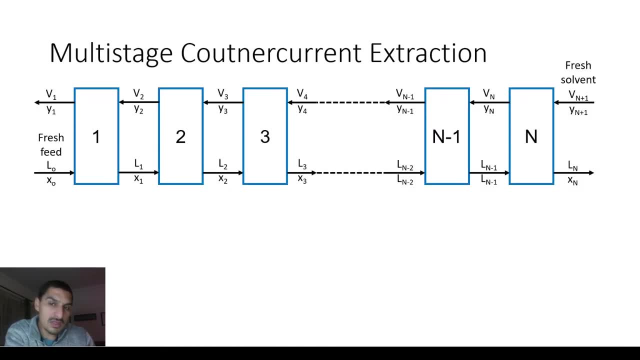 and and recover it. so it's not practical to use a single stage, even if you use a large amount of solvent. it's not going to be economical and that's why we use the what we call the multi-stage, etc. I'm using many stages, Like we do in distillation. 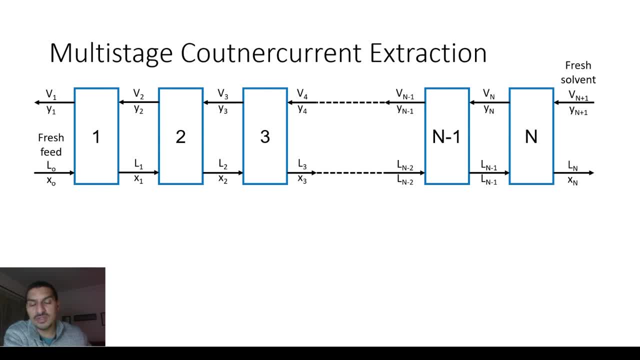 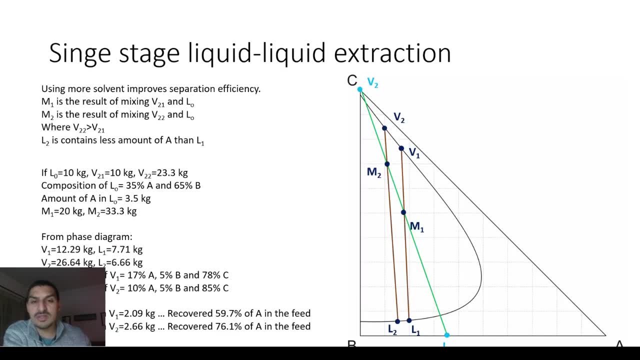 Like we do in all Mass transfer operations. So this is Going to be the topic of the next video. We're going to see exactly Like we did today. We'll see the equations And we'll see How we apply this graphically. It's going to be a little.